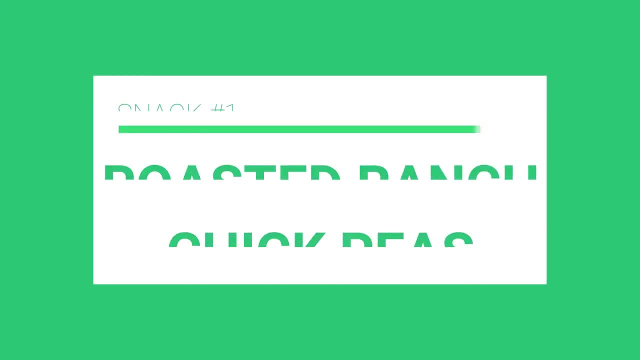 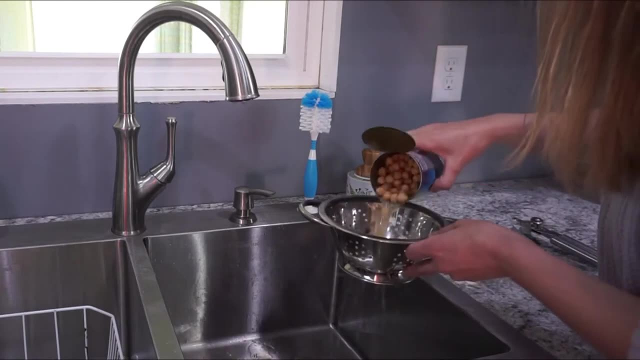 hit, subscribe and we'll get right into the snacks. For this recipe, you're just going to need a can of garbanzo beans that will be drained and rinsed, and then you'll also need a packet of ranch seasoning, So go ahead and preheat. 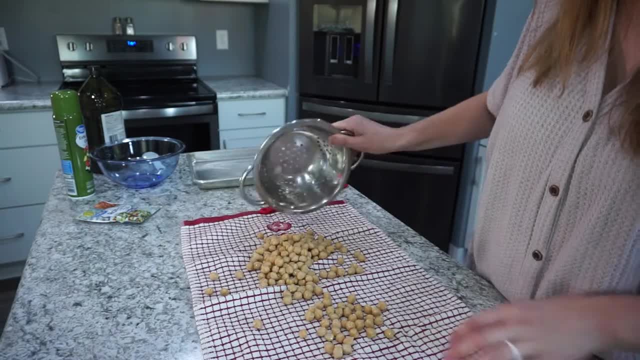 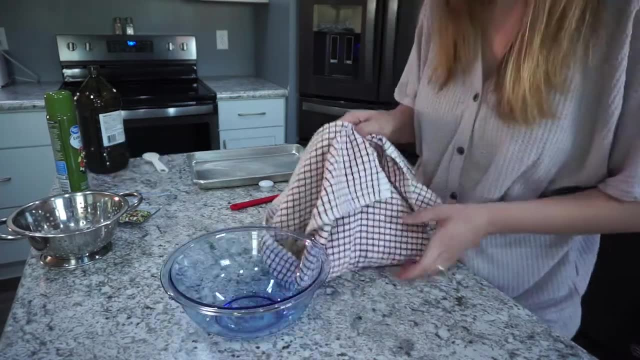 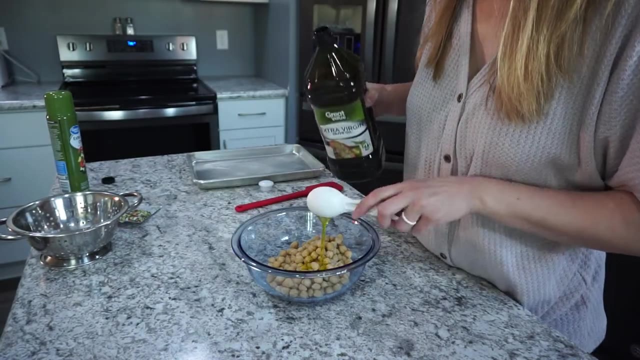 your oven to 400 degrees and then we're just going to be drying off the garbanzo beans. Just be really gentle so they don't break or anything. Once the beans are dry, go ahead and place them in a bowl, and then we're going to be adding a tablespoon of oil and 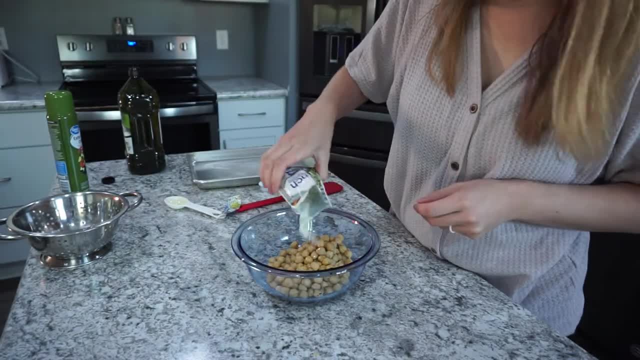 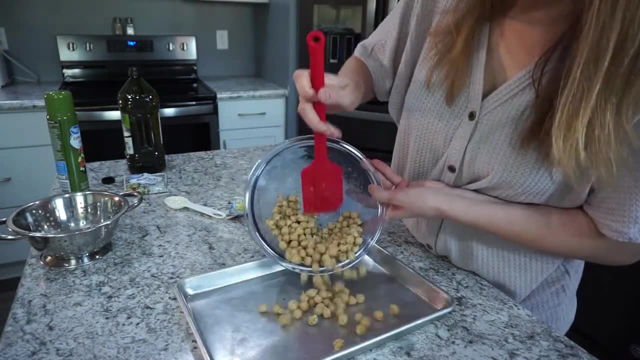 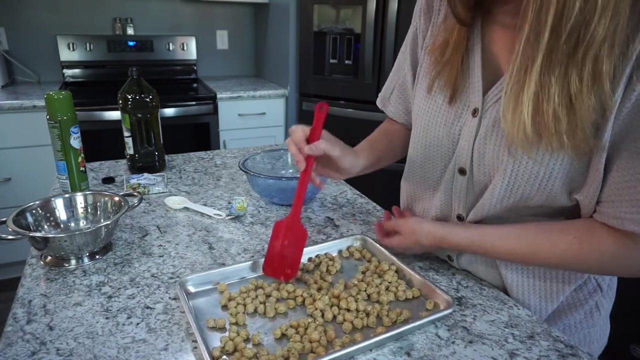 half a packet of ranch seasoning mix, And then you're just going to go ahead and mix that all together, Place your beans onto a baking sheet, and then you're just going to want to spread them around evenly so that they are baked all the way through Place. 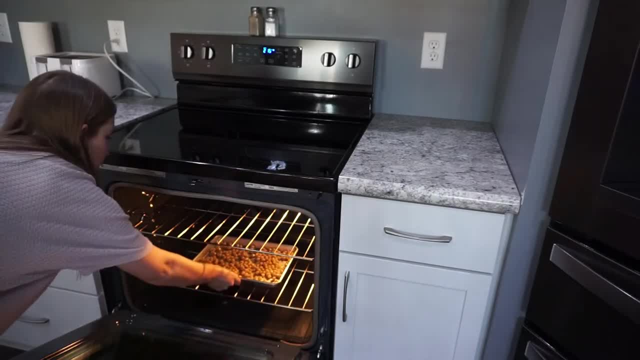 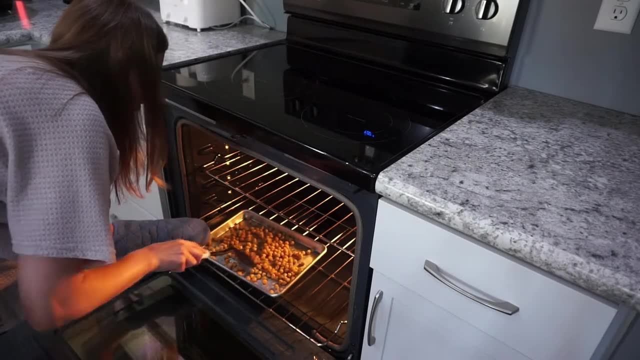 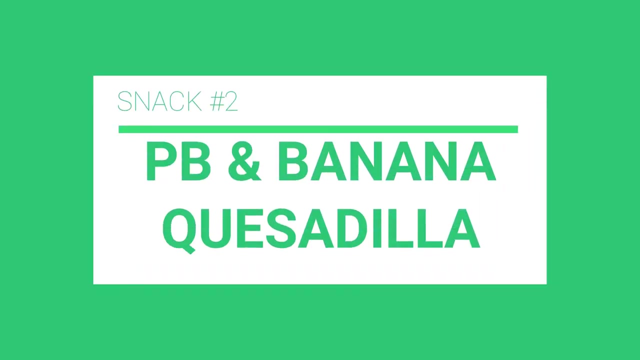 them into the oven and then we're going to be wanting to stir them about every minute, Every 10 minutes. Mine took about 40 minutes to roast, but you're going to want to roast them until they're nice and crunchy and golden brown. This next recipe is super simple. You're 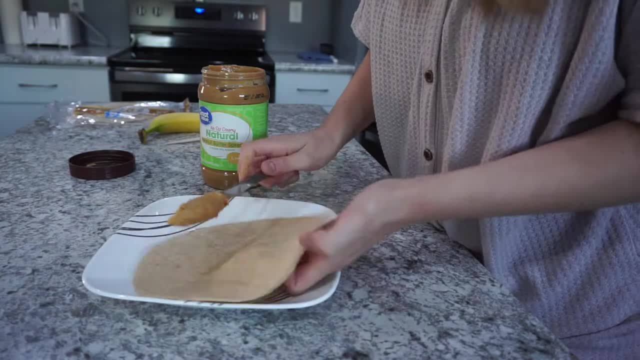 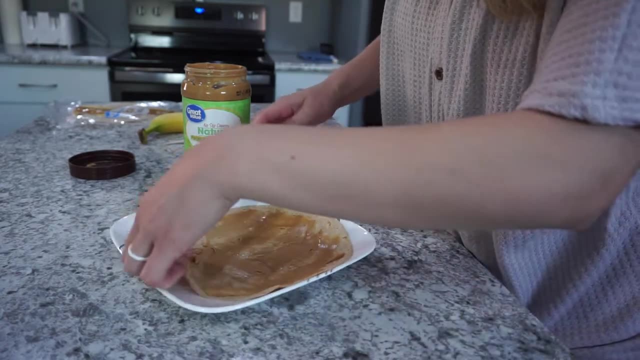 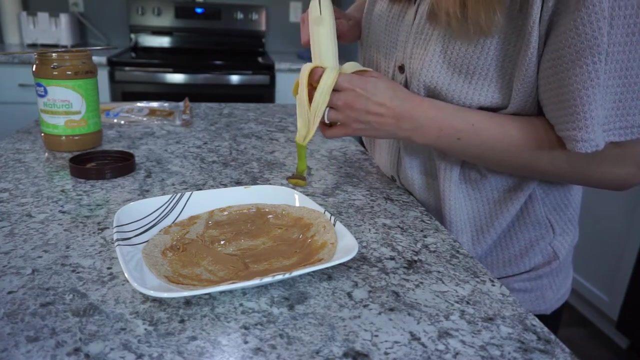 just going to take a wheat tortilla and then add some peanut butter to that And then just take a banana and put some slices on there. I like to split my banana in half first, just because for my son- he's a toddler and I want to make sure that it is not a choking. 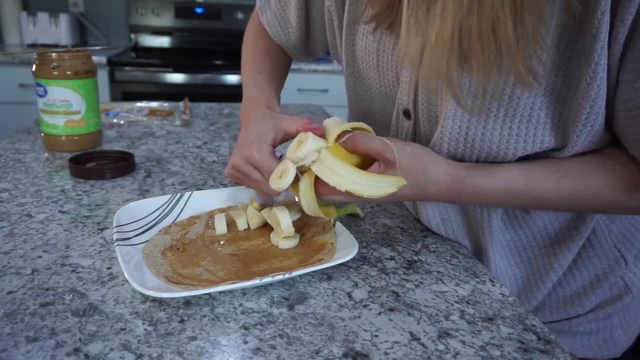 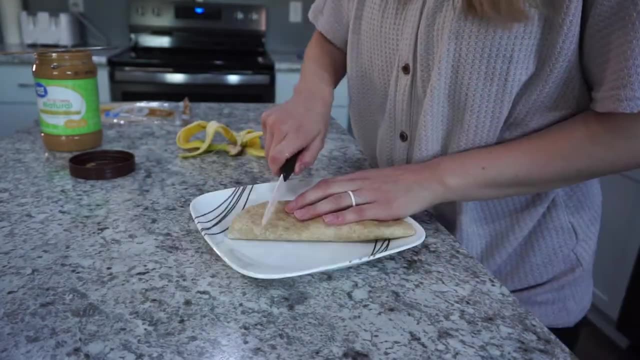 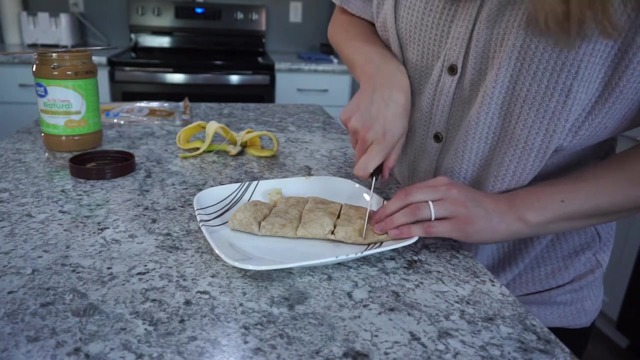 hazard for him. So I want to make the pieces nice and small, And then I just cut this up into strips and serve it to him, And he loves this for breakfast, lunch or for a snack, so it's a really good one for him. 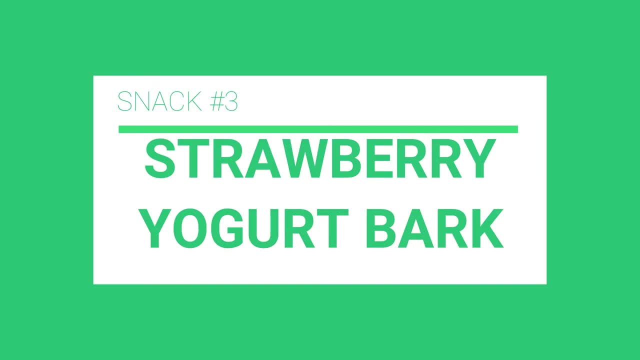 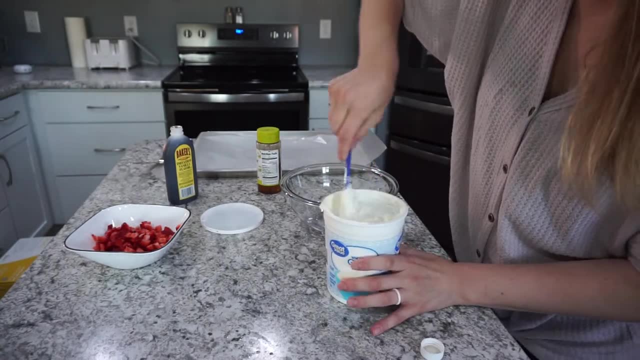 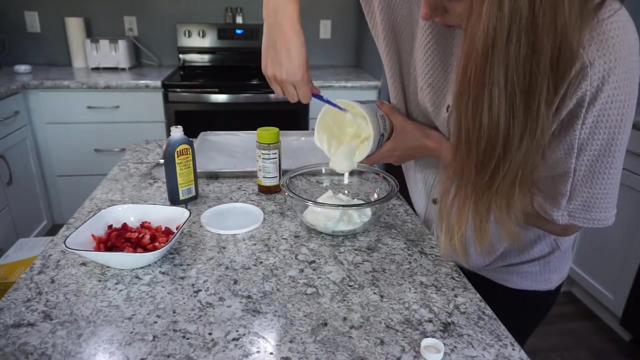 For the yogurt bark. I like to use whole milk yogurt, just because my son is only one, so I like to give him the extra fat and the calories. So just add however much you want into a bowl. I like to use almost the full container of Greek yogurt and then I leave a little bit. 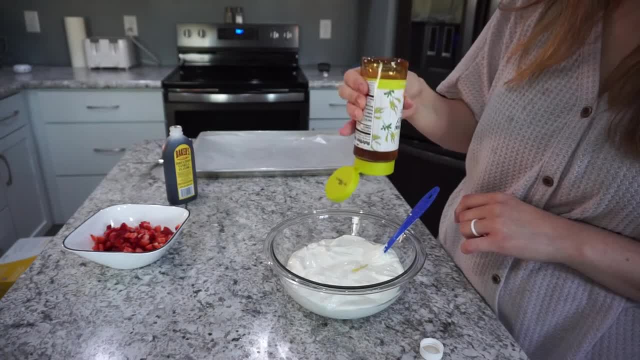 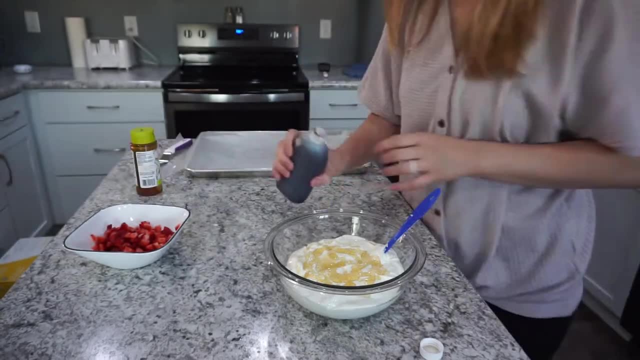 in there, And then I like to add honey and vanilla to mine, but you could really add whatever you like. The options are endless. You could do melted peanut butter or chocolate chips or really whatever you want. So just mix that all together. 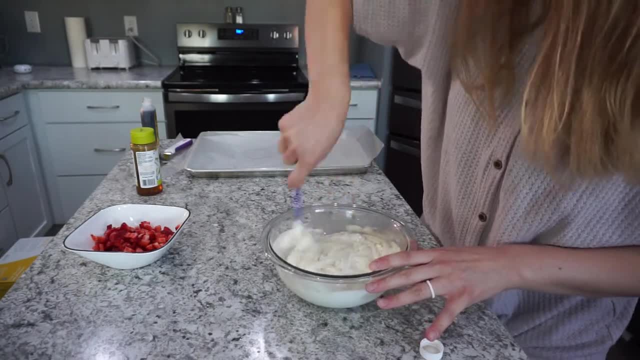 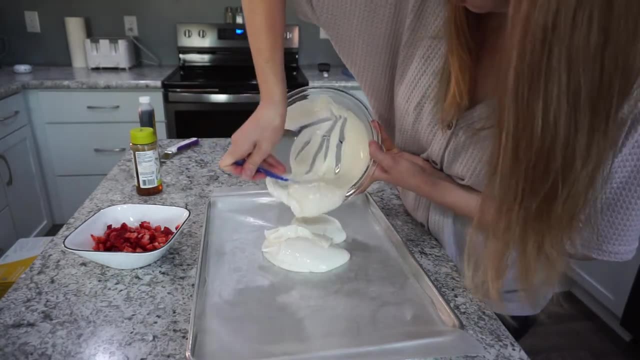 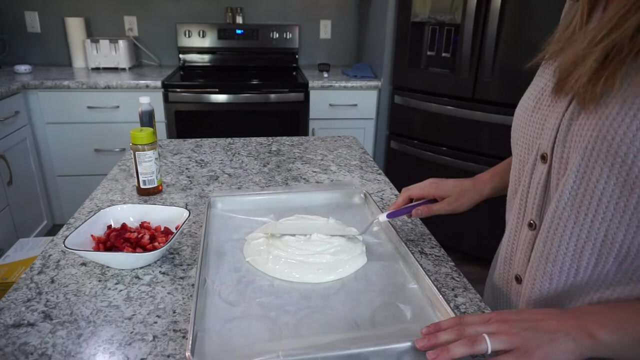 And then add that onto a lined baking sheet. I used wax paper. Parchment paper works as well, but you're going to want to use something so you're able to get the yogurt bark off of that after we put it in the freezer. I'm using a frosting spatula to spread mine around. 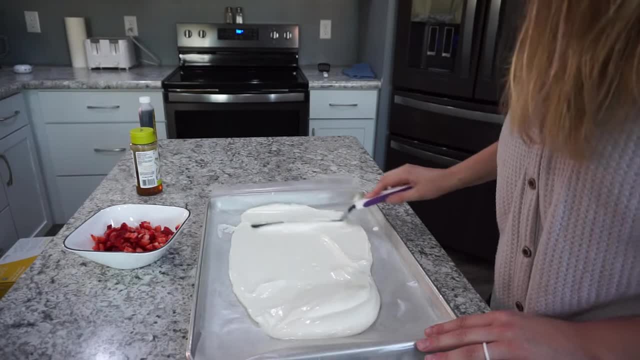 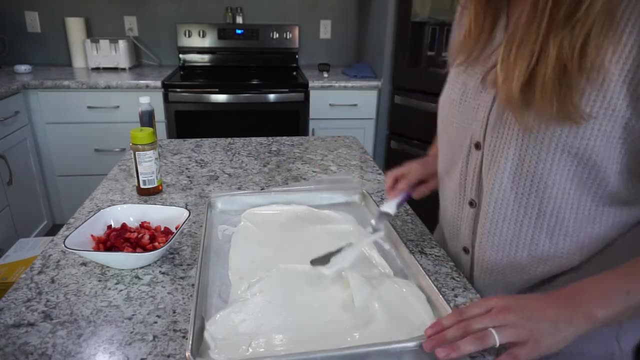 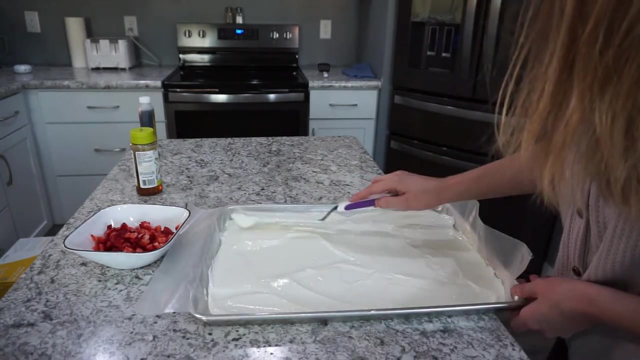 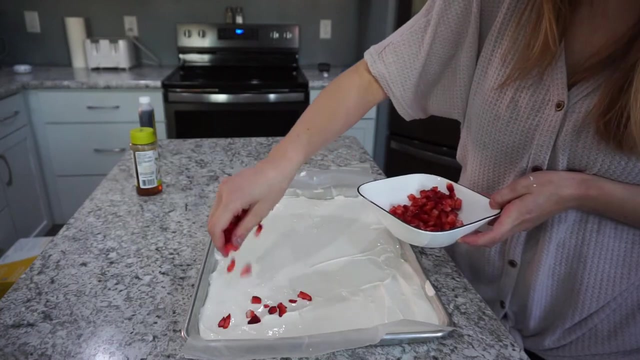 I just think it works really well. It makes it nice and smooth and it just works very, very well. But you could definitely use just a spoon or a knife or anything that you have on hand. On this particular day, I decided to top mine with strawberries, but we also really like 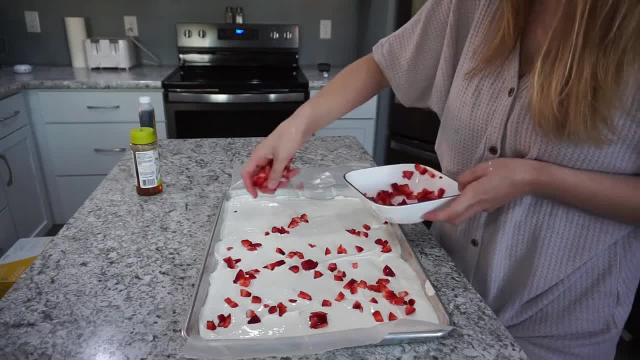 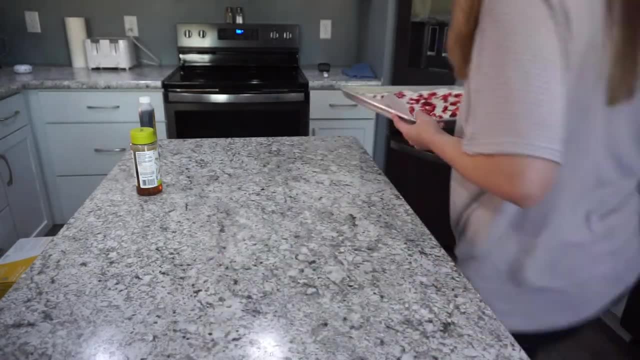 like peaches or really any kind of fruit. Peanut butter's really good, You know. I really good mix throughout this and we really like that as well. go ahead and stick that in the freezer for about an hour to two hours, just until it really sets. 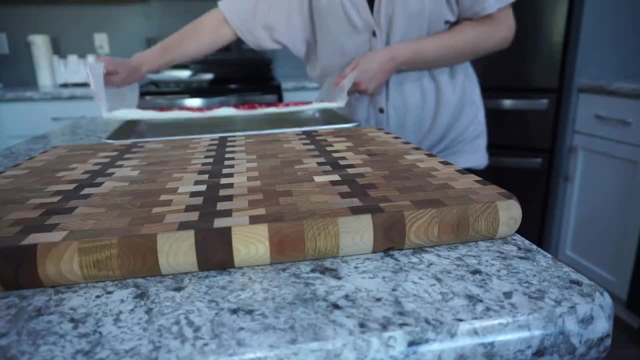 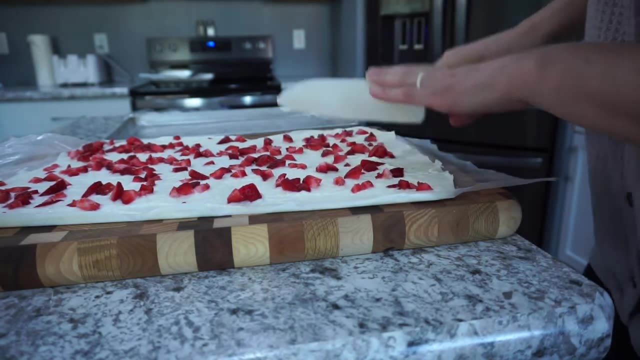 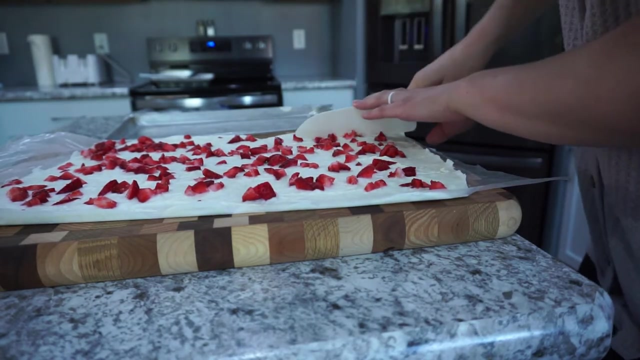 firmly and then, once it's done, you're just gonna take it out and cut it and it'll make nice little squares of yogurt bark. this is so nice for snacks or for breakfast. my son really enjoys it and it's way less messy than giving him regular yogurt. 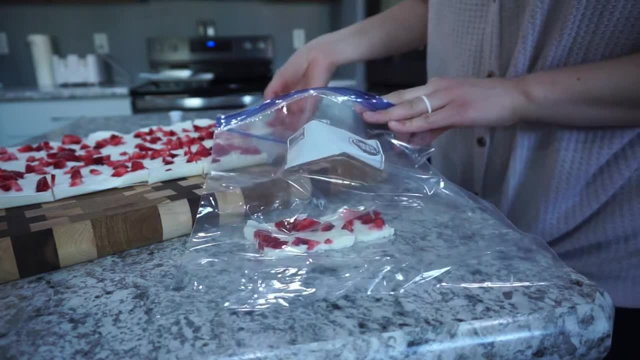 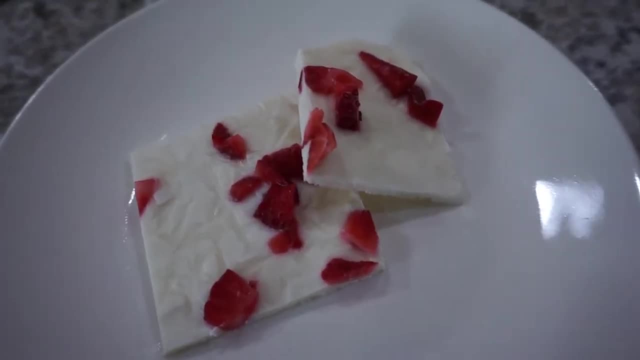 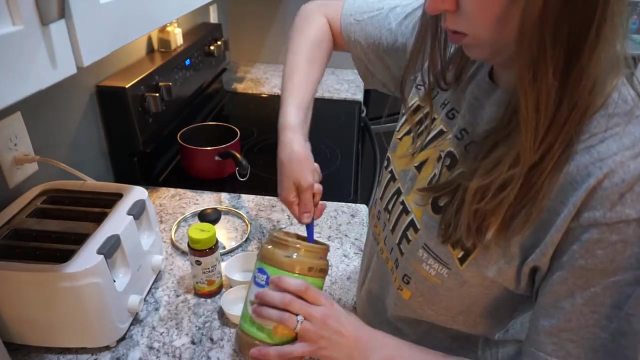 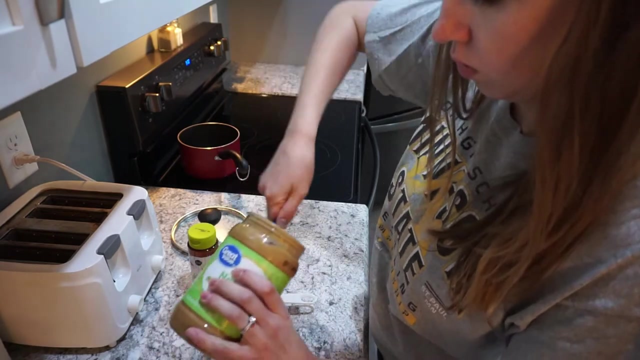 obviously you're just gonna want to store this one in the freezer, and that is it for this recipe. these cheerio snack bars are super simple and easy and my son really enjoyed them, and they only have three ingredients, which is very, very nice. so I'm taking 3 quarters of a cup of natural peanut butter, and then I'm also. 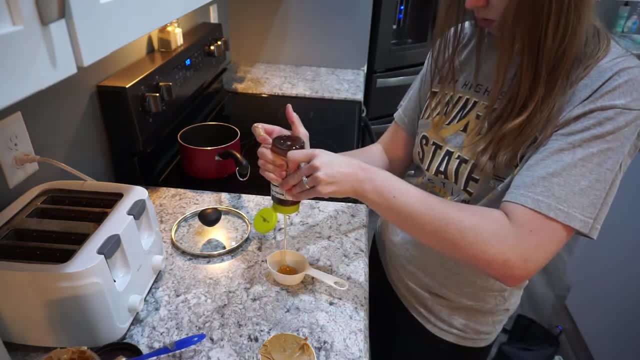 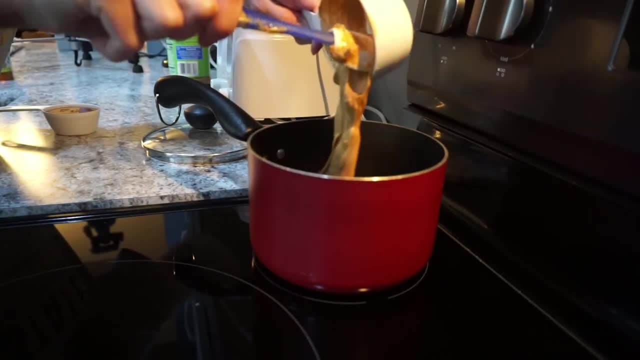 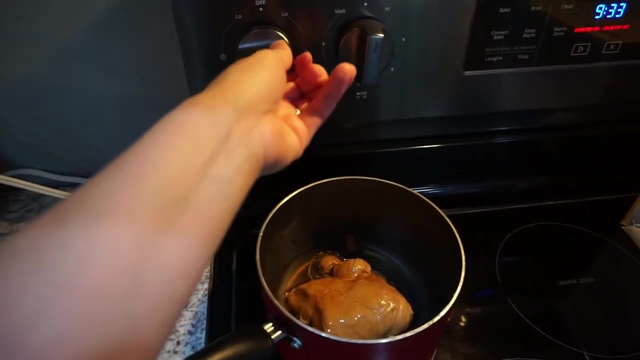 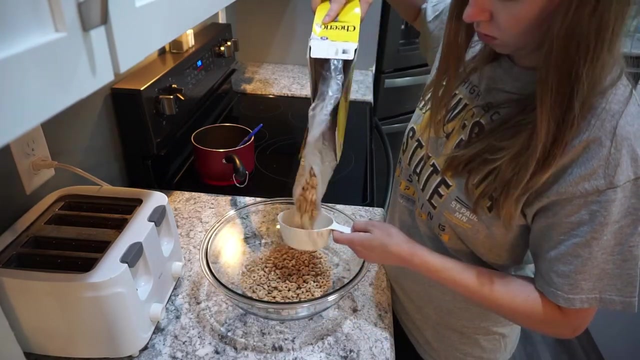 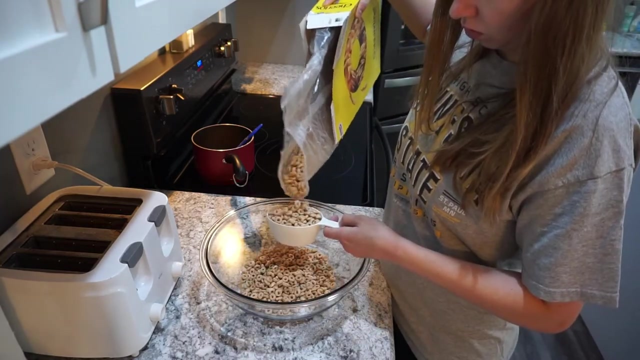 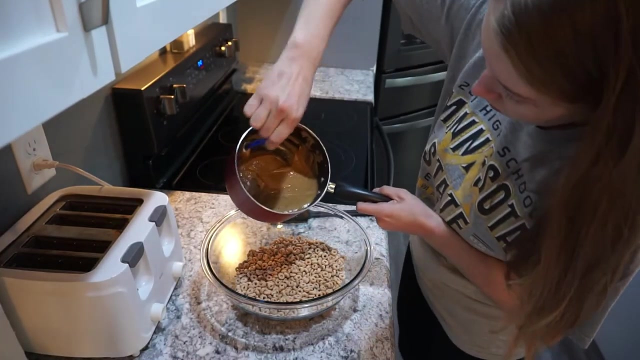 gonna do half a cup of honey and you're just gonna melt those together in a saucepan on medium heat, you, you- and then add the peanut butter and honey mixture right over top of the cheerios and mix it all together and then add the peanut butter and honey mixture right over top of the cheerios. 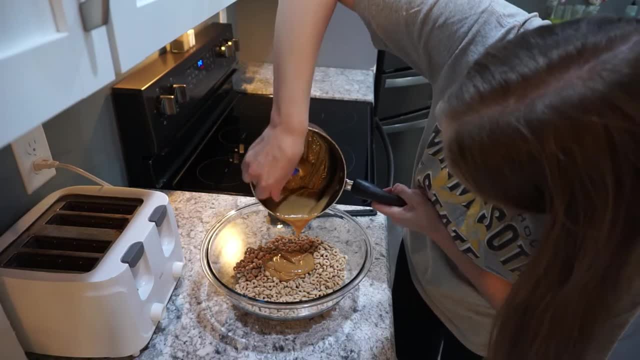 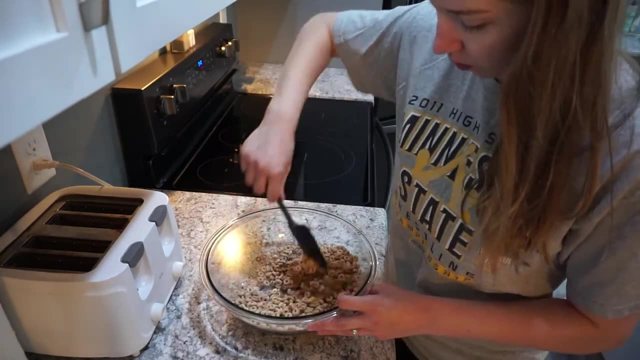 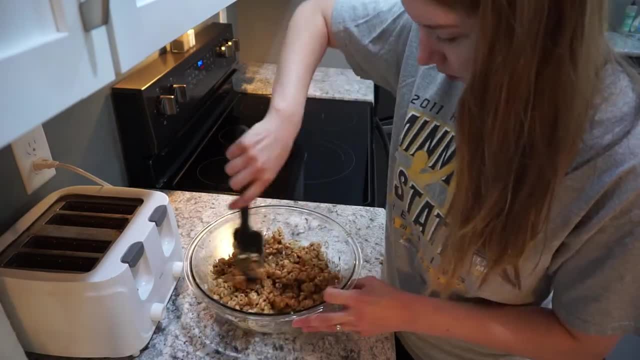 and mix it all together. and then add the peanut butter and honey mixture right over top of the cheerios and mix it all together. and then add the peanut butter and honey mixture right over top of the cheerios and then add the peanut butter and honey mixture right over top of the cheerios. 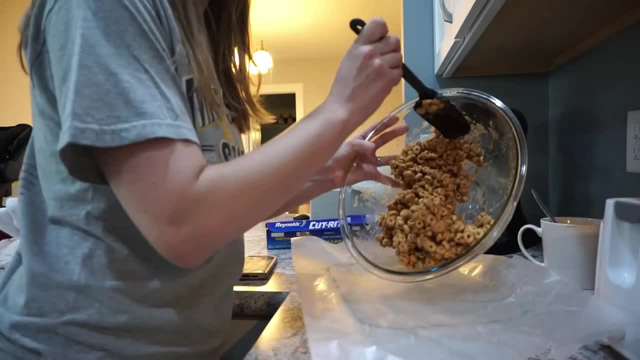 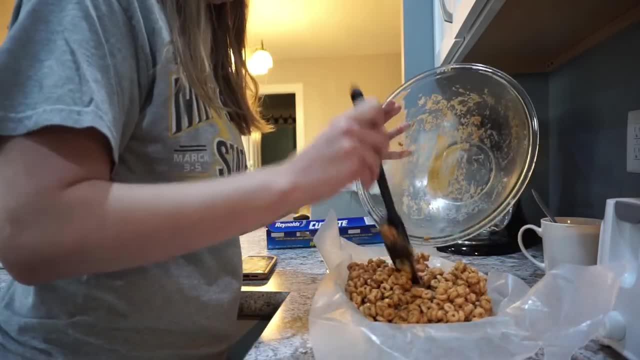 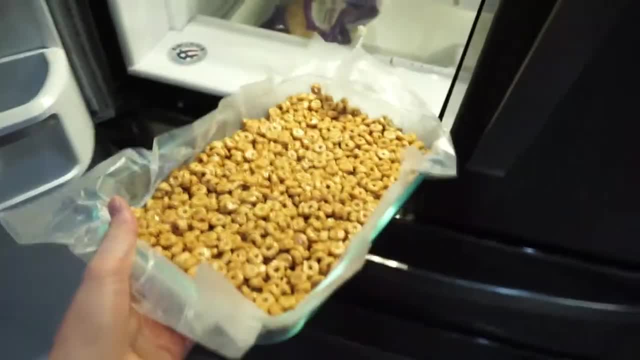 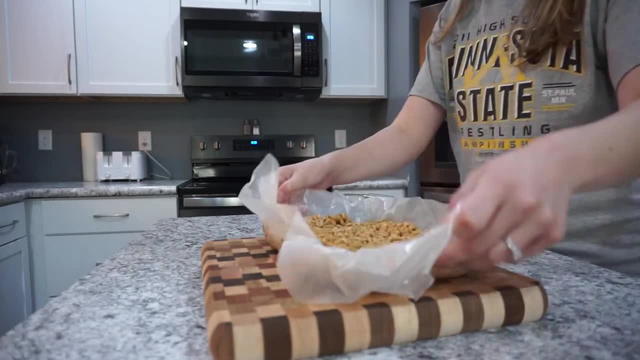 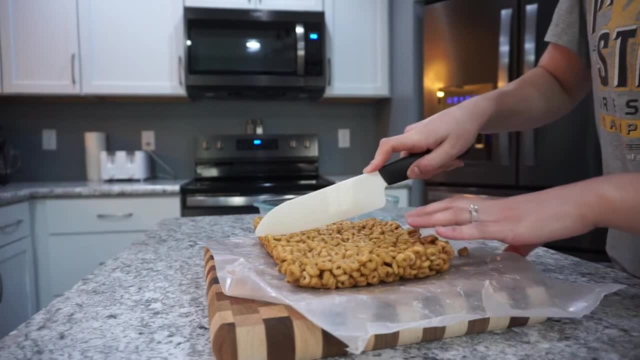 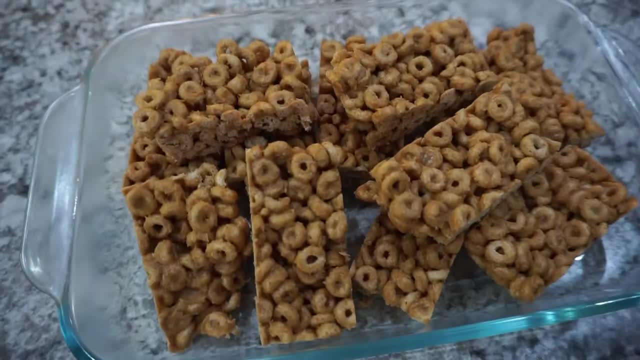 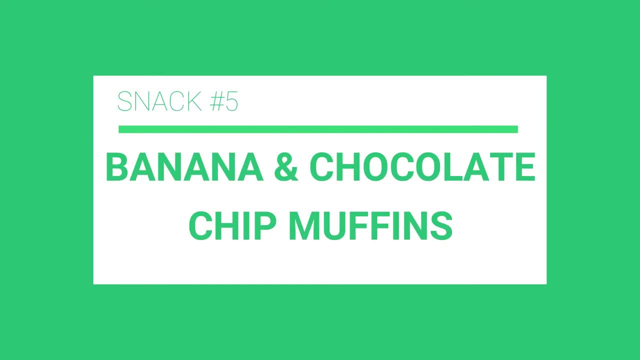 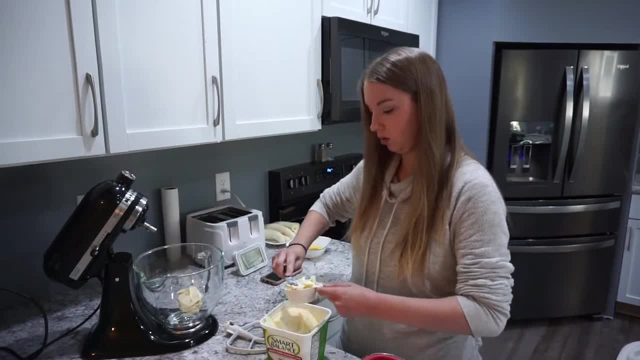 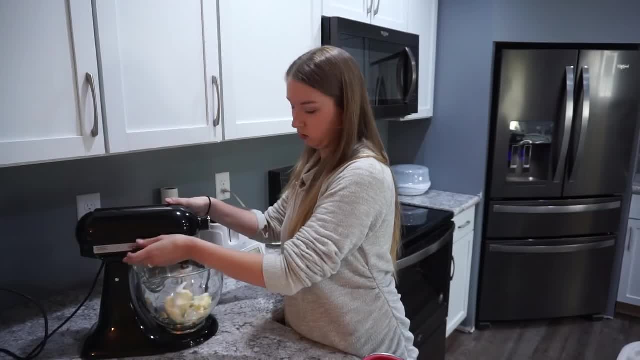 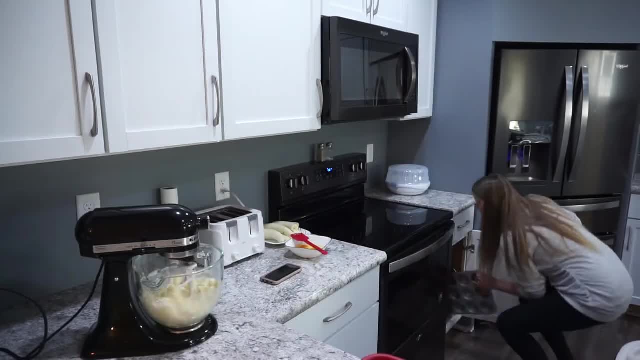 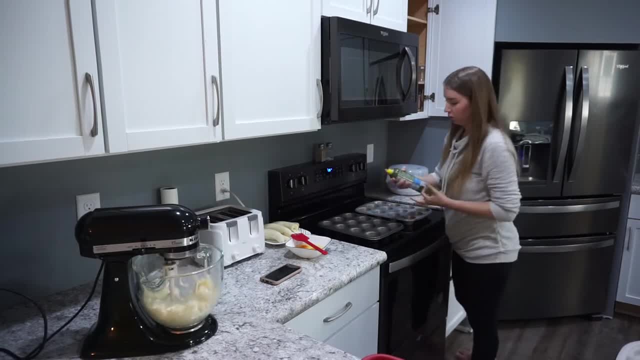 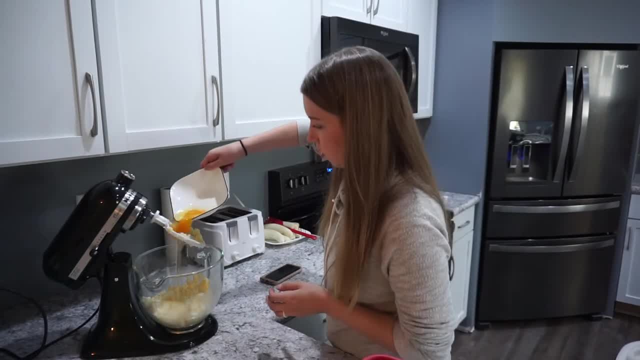 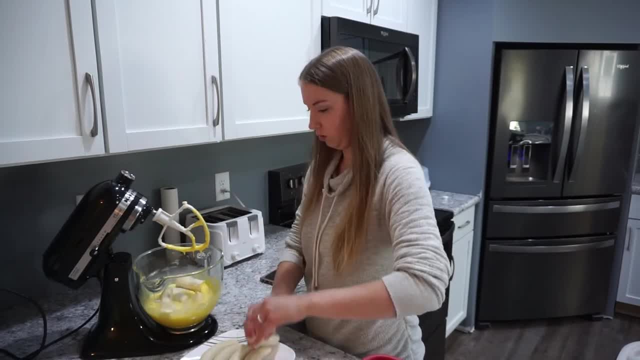 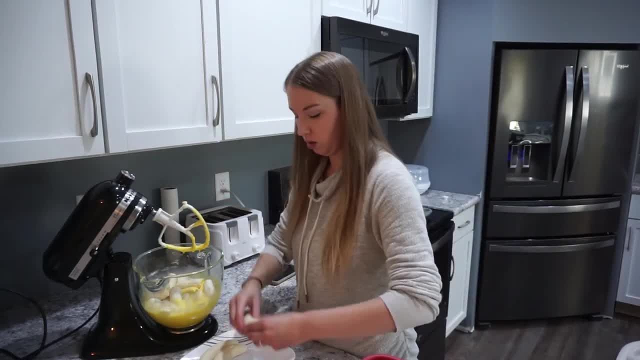 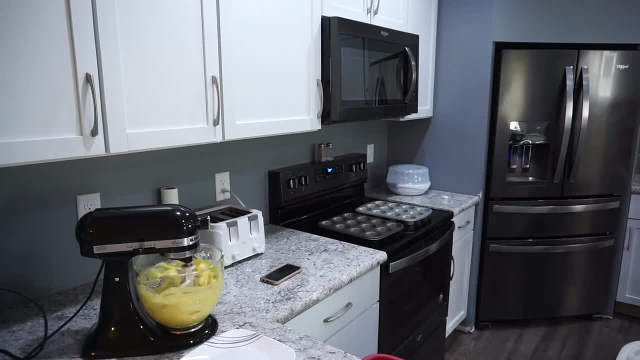 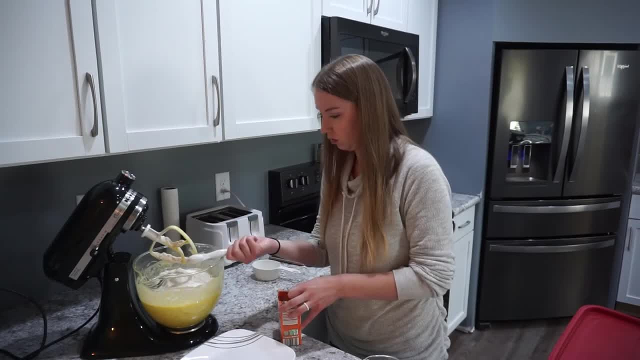 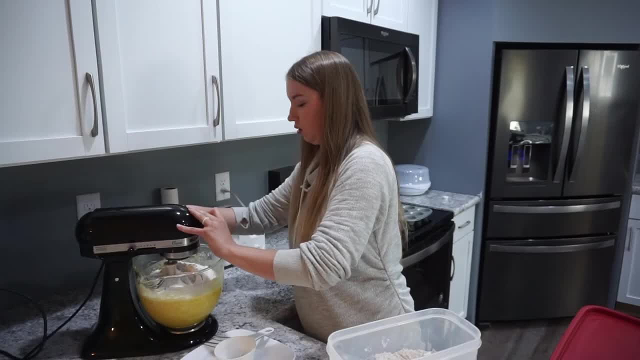 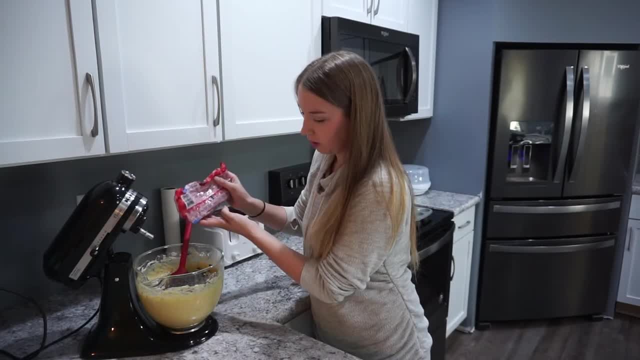 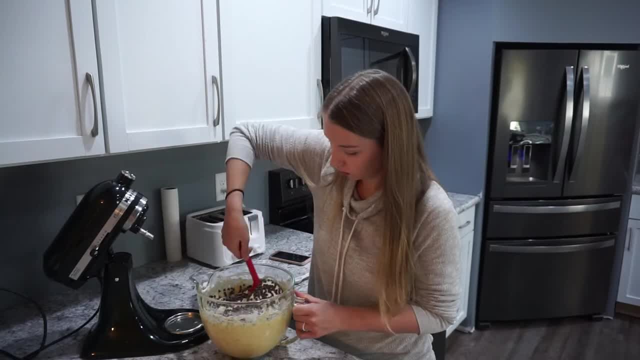 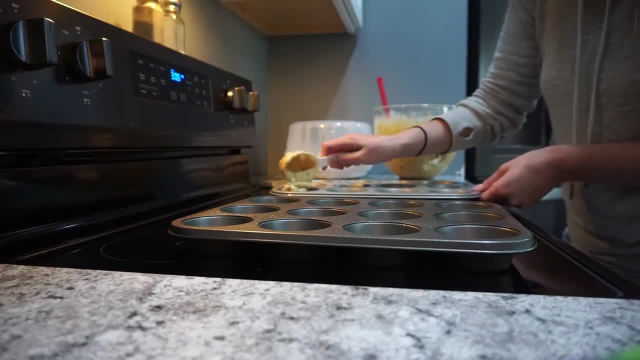 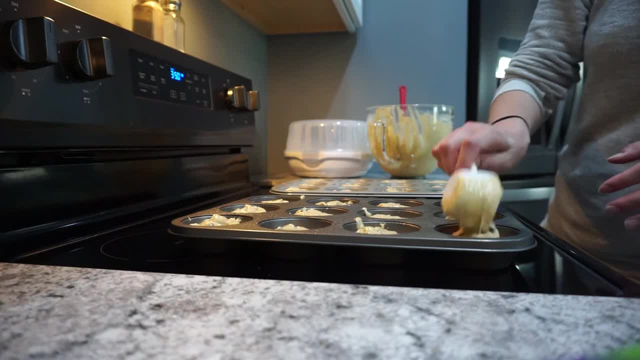 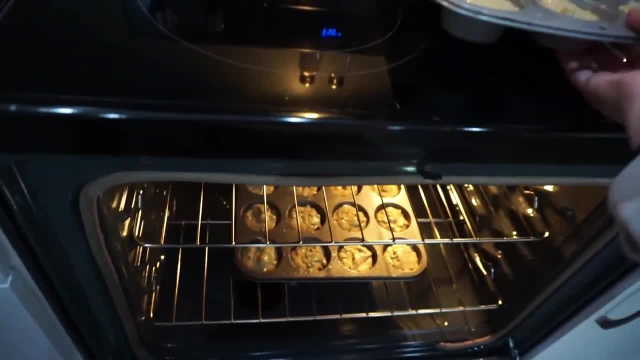 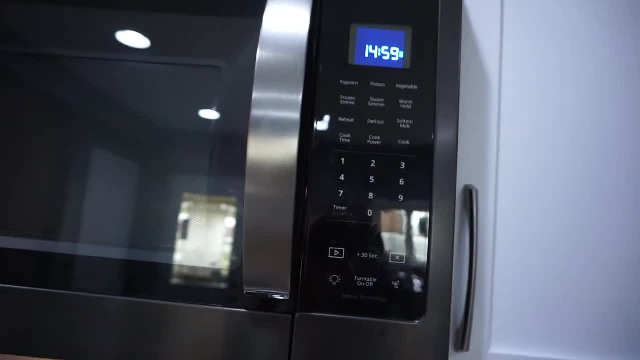 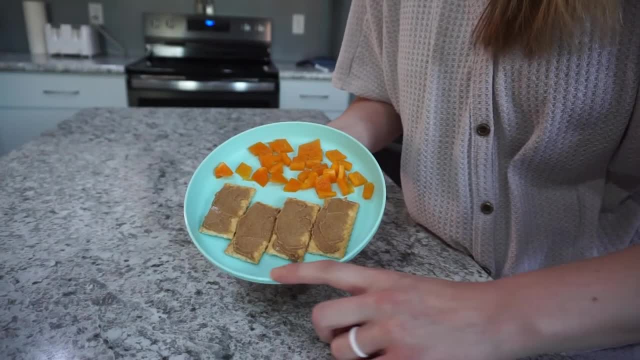 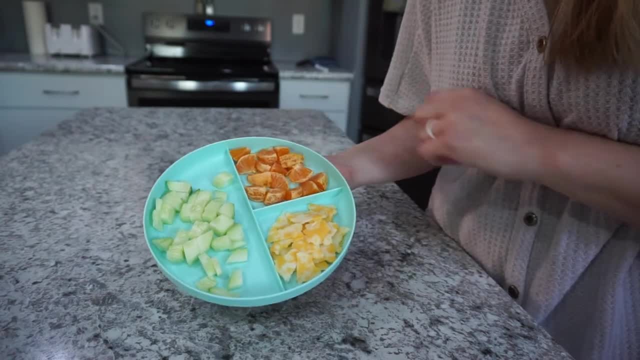